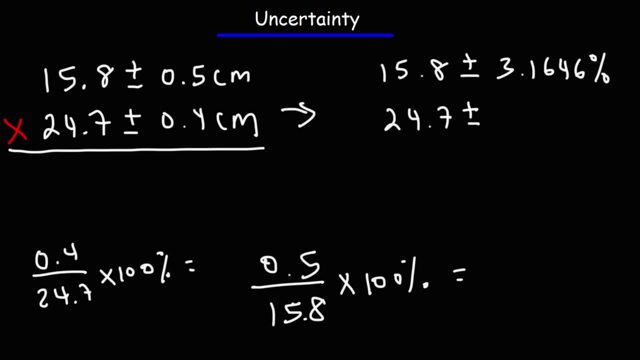 So that's going to be 1.6194.. All right, so now we're going to multiply these two numbers. So let's use a calculator to multiply 15.8 and 24.7.. So that's going to be 390.26.. 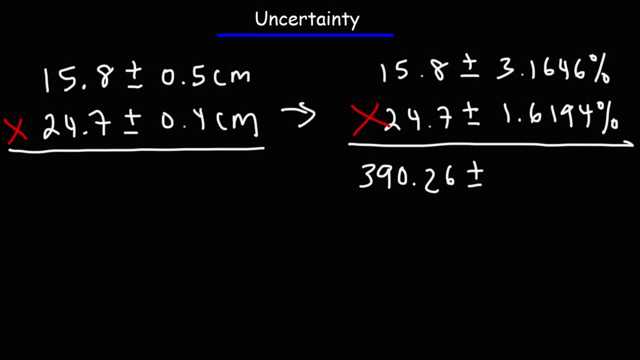 Now for the uncertainties. we're going to add them, We're not going to multiply them. For this to work, you need to add the percentages, So 3.1646 plus 1.6194, that's going to be 4.784%. 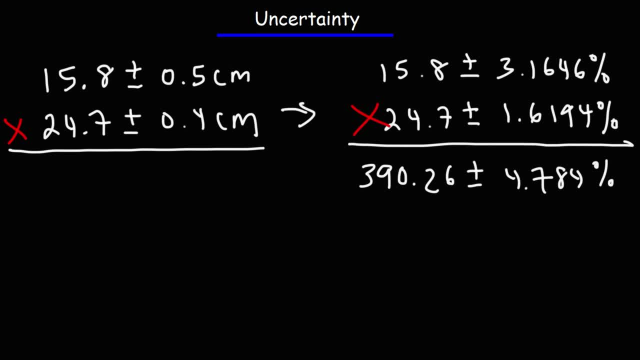 Now there's still some other things we need to do. So now that we have the percentage, we need to convert it back into a non-percentage form. So what we need to do is find out what is 4.784% of 390.26?. 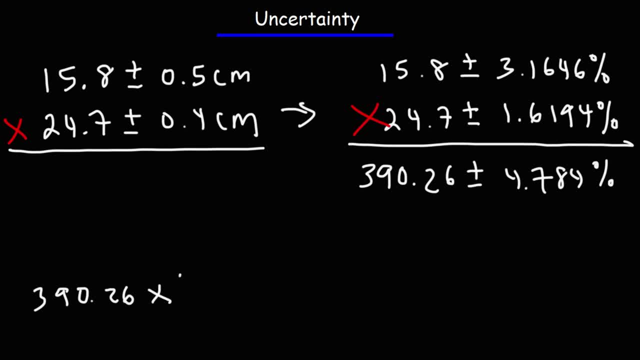 To figure that out: take 390.26,, multiply it by this value as a decimal. If you take 4.784% and divide it by 100, the decimal value is 0.04784.. Basically, move the decimal two units to the left. 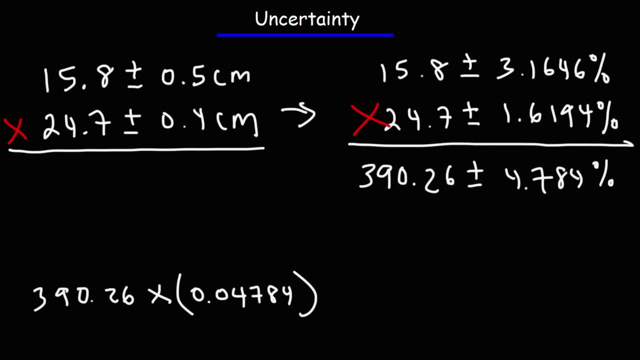 So 390.26 times that number will give us 18.67.. So we have 390.26 plus 18.67 as our answer. But now let's round it to the appropriate number of significant figures. So, looking at our original numbers, 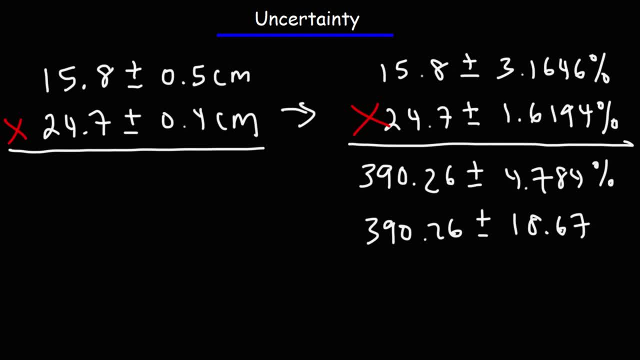 we see that they have three significant figures. So to round 390.26 to three significant figures, we could say it's simply 390, with the decimal point which will make the zero significant. Now, looking at our uncertainty: the 0.5 or the 0.4,. 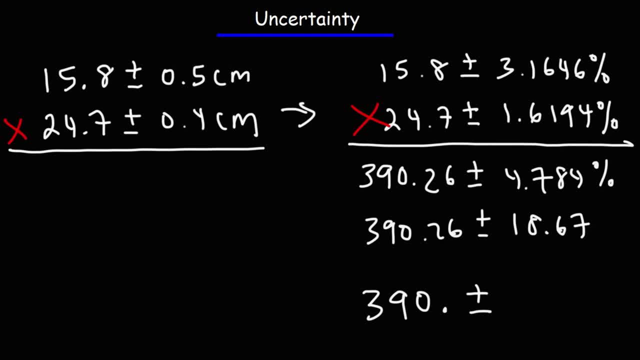 it only has one significant digit. So let's round 18.67 to a number with one significant digit, and that's going to be 20 without a decimal point. So the zero is not significant. And then we need to put the unit centimeters. 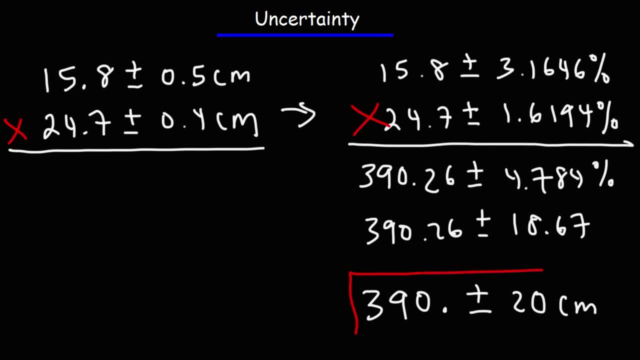 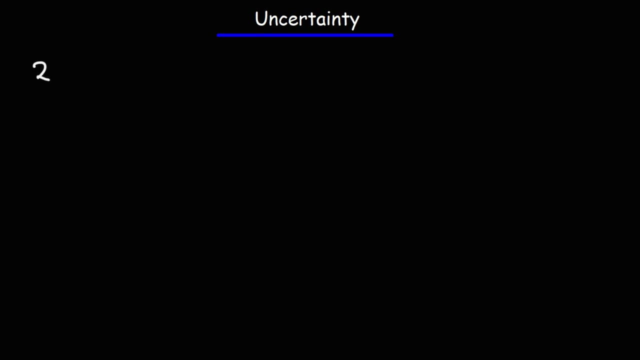 So this is the answer for this problem. So now you know how to multiply two numbers that contain uncertainty values. Now let's try an example with division. So let's say we have this number, 28.4 plus or minus 0.6 centimeters. 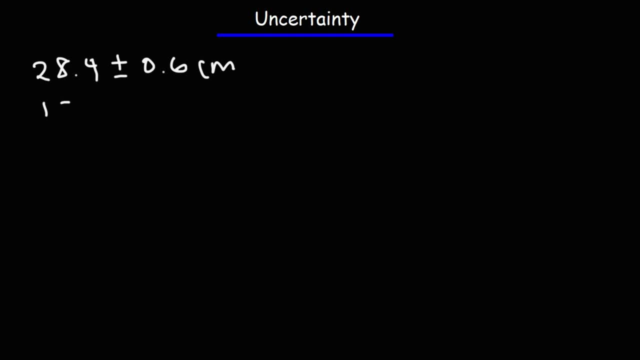 And the next number is going to be 15.2 plus or minus 0.6.. So this number is going to be 15.3 centimeters. So this time we're going to use division. We're going to divide the top number by the bottom number. 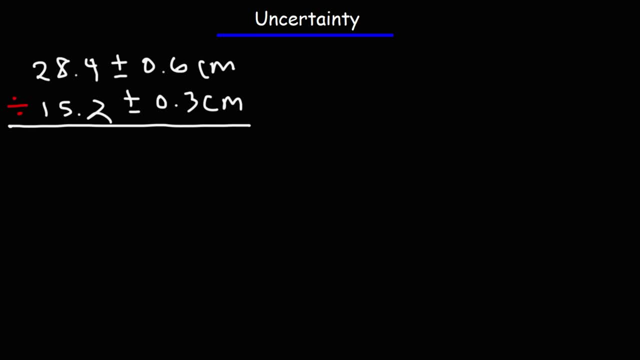 But now, just like before, we need to convert the uncertainty into a percentage value, or we need to get the percent uncertainty. So let's start with the top number. It's going to be 0.6 divided by 28.4 times 100%. 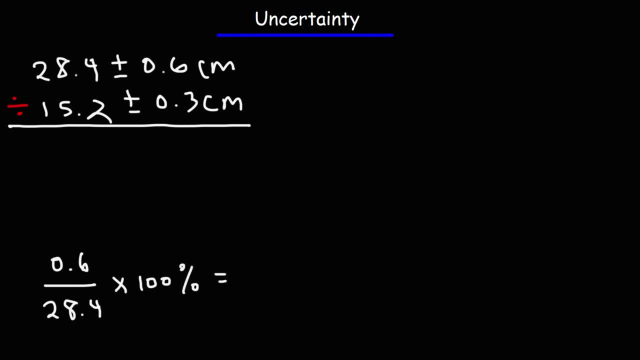 So 0.6 times 100 is 60.. 60 divided by 28.4.. That's 2.1127%. Now let's do the same thing with the other number. So we're going to take 0.3,. 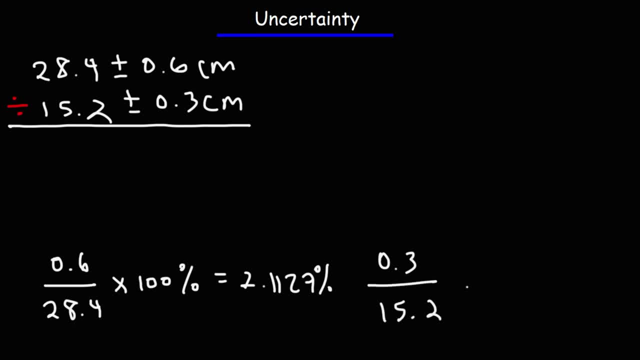 and we're going to divide it by 15.2, and then multiply that by 100%. So 0.3 times 100 is 30.. 30 divided by 15.2.. That is going to give us 1.9737%. 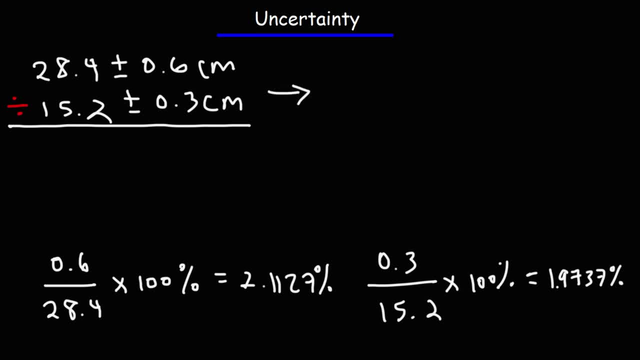 Now let's rewrite the problem. So this is going to be 28.4 plus or minus 2.1127%, And then the bottom number, 15.2.. Plus or minus 1.9737%, And we're still dealing with division. 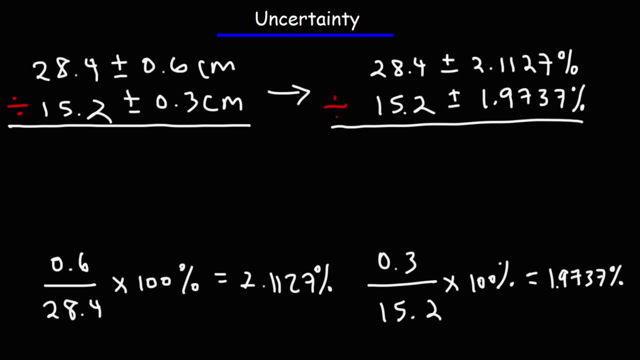 All right, so now we can get rid of this: 28.4 divided by 15.2.. So that's 1.8684.. I like to get a few additional digits because I'm going to round it later, And plus, I'm going to get a percentage of that number. 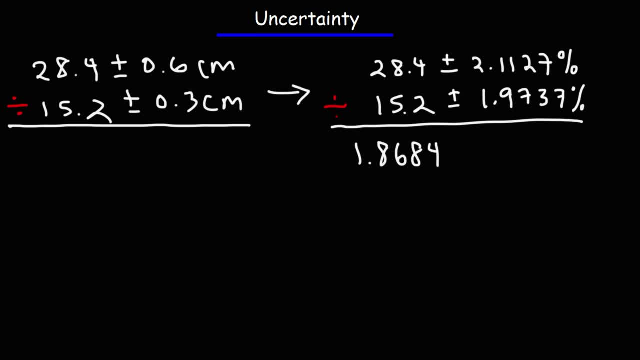 So I want to get a more accurate answer and then round at the very end. When you round in the middle of the operations it'll compound and create a bigger error at your final answer. So it's always good to round at the very end. 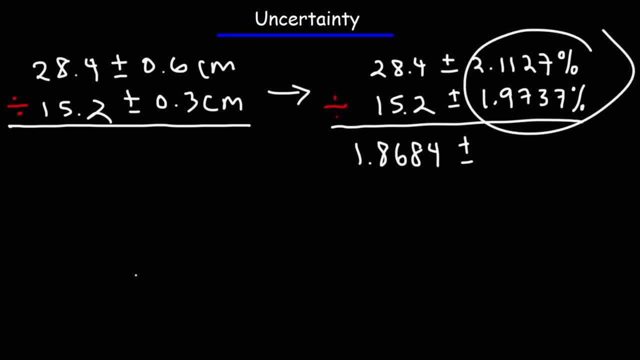 So now let's add the two percentages, just like we did before. So the rules for multiplication and division are the same. You need to convert the uncertainty into a percent uncertainty And then, when you perform the operation, be it multiplication or division, 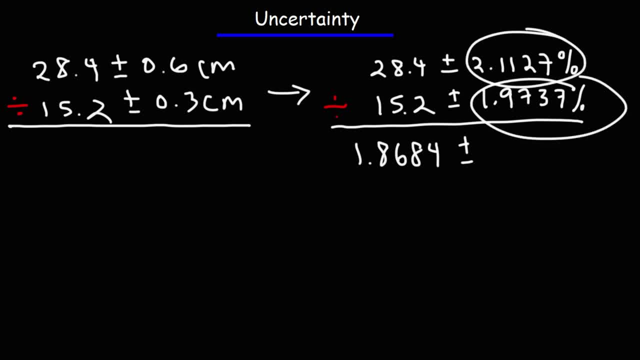 in both cases you need to add the percent uncertainty: 2.1127 plus 1.9737.. That is going to be 4.017.. So what is 4.064%? All right, So now that we've done the operation. 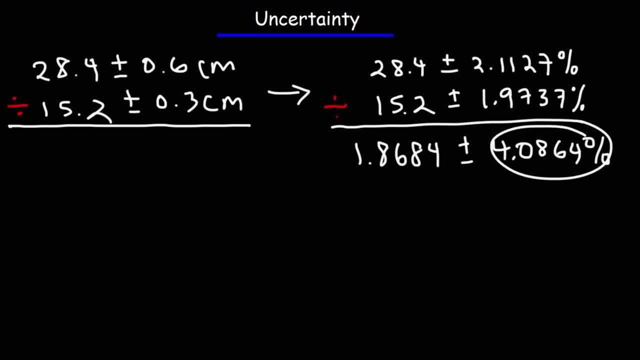 let's convert the percent uncertainty into a non-percentage uncertainty value. So what is 4.0864% of that number? 1.8684? That's going to be 1.8684 times 4.0864.. 4.0864.. 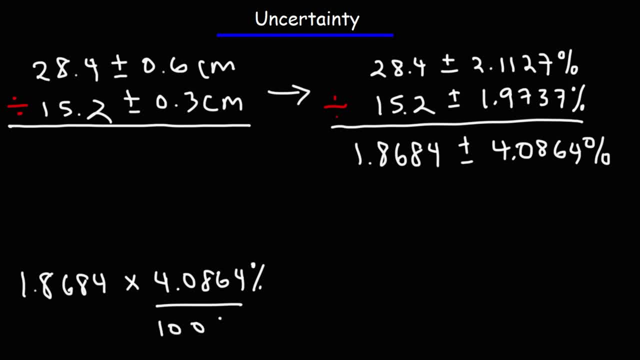 4.0864.. 4.0864. 4.0864. 4.0864.. 4% times divided by 100%. So this works out to be .07635.. So this is going to be 1.8684.